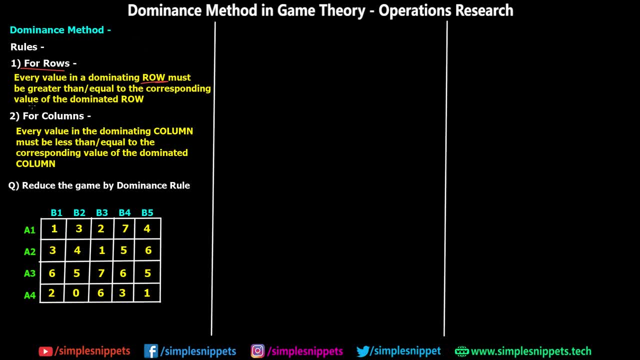 row must be greater than or equal to the corresponding value of the dominated row. And the second rule is for columns and it goes as follows. So every value in the dominating column must be less than or equal to the corresponding value of the dominated column. So basically, 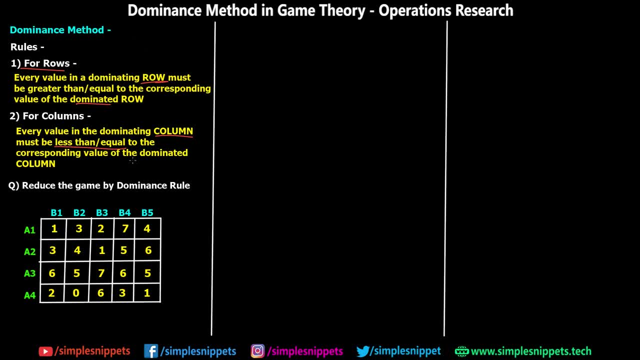 what this Dominance Method helps us achieve is it helps us reduce the payoff matrix into lesser number of rows and columns, so that the problem gets solved. So sometimes what happens is in some numericals we do not get the saddle point using the Maximin. 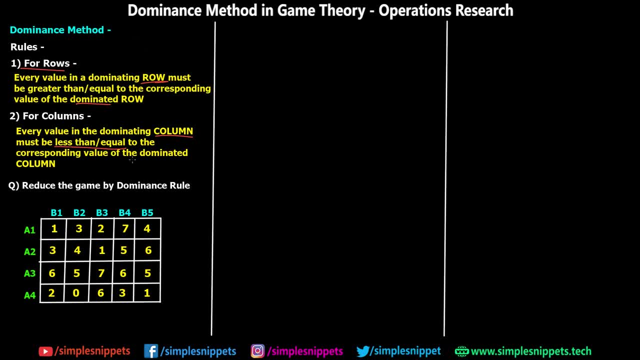 and Minimax method, and then we have a mixed game in that situation. right, We've seen that in the previous videos, wherein we saw the difference between a mixed game and a pure strategy, and we also saw examples on pure strategy. So if you've missed those videos, 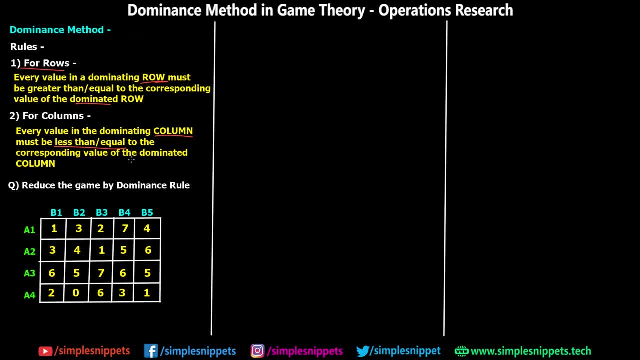 you can check it out. But what this Dominance Rule basically, as I mentioned, does is, it helps us to reduce the payoff matrix to a simplified version. So in this question you can see the payoff matrix wherein we have player A and player B, So the blue ones is player. 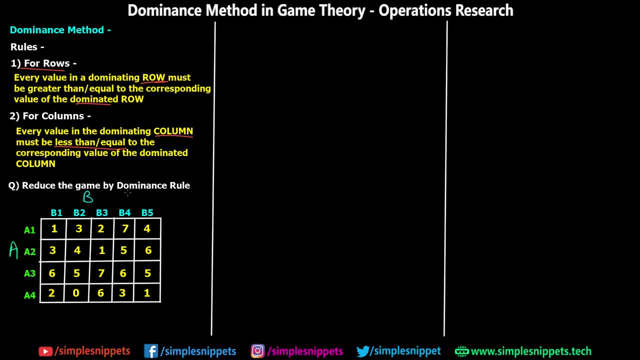 B and the green one is player A, and we have to reduce the game by using Dominance Rule. Now you can use the Maximin and Minimax method on this payoff matrix as of now and you'll get the saddle point. So this, in this numerical, it's a kind of pure strategy game, But we 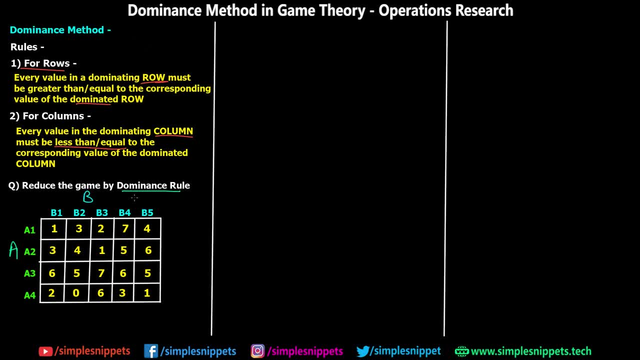 are going to be using the Dominance Rule to see how this entire numerical goes. Okay, so we are going to be applying these two rules on this payoff matrix to reduce it to a smaller matrix, and as we reduce it to smaller, smaller chunks, we'll finally achieve the final answer. 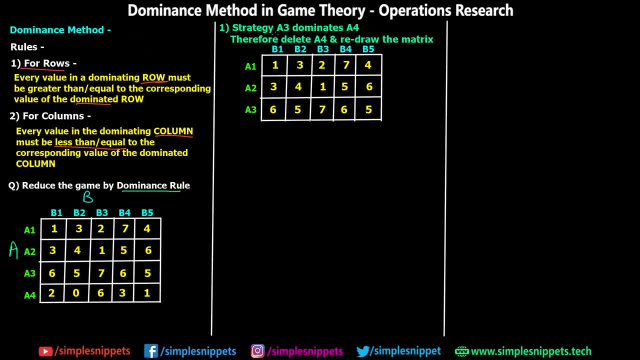 So let's see how that works. Okay, so in step number one we say: strategy A3 dominates strategy A4. Therefore, delete A4 and redraw the matrix. So what did we do over here? So we use the rules which are applied for the row and for the row. the rule is: every value in the dominating. 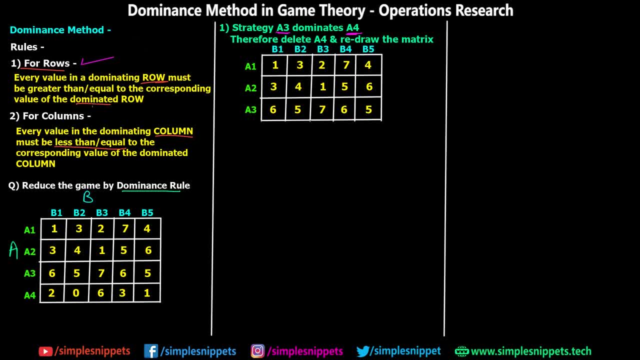 row must be greater than or equal to the corresponding value of the dominated row. So when we are talking about A3.. In A4, we are talking about these two rows, right? So in the question we have these two rows. Now, according to the rule, what is being said is: A3 dominates A4.. So the 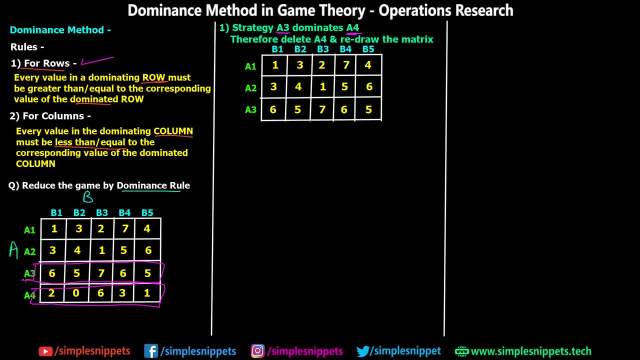 reason why A3 dominates A4 is because every value in A3, that is, 6,, 5,, 7,, 6, 5, is greater than or equal to every value in A4. You can see, 6 is greater than 2, 5 is greater than. 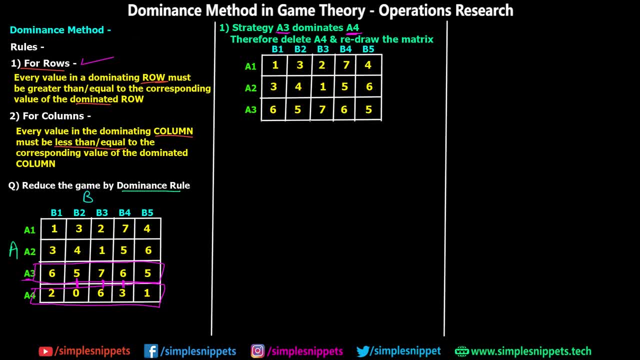 0,, 7 is greater than 6,, 6 is greater than 3,, 5 is greater than 1.. So our first rule applies over here. So we have taken B4.. We delete A4 and redraw the matrix. So we completely delete this. 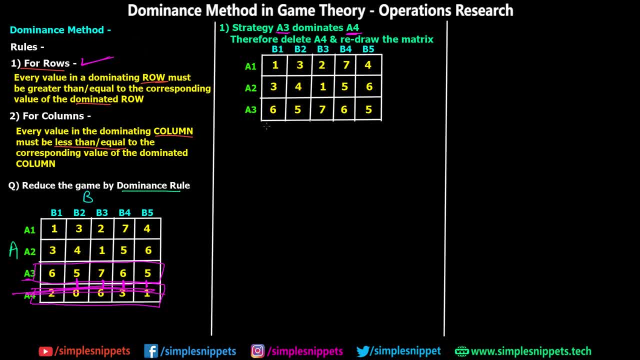 entire row A4 and we redraw a new matrix wherein we do not have A4.. So for player A, we have just removed the strategy A4.. So this is step number 1.. Let us see what is step number 2.. So in step number 2, what we say is: strategy B1 dominates B4. therefore, delete B4 and redraw. 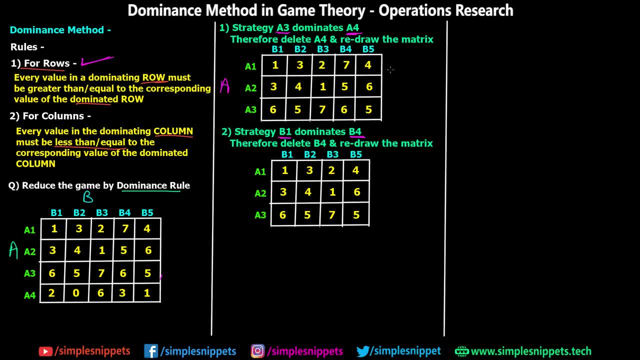 the matrix. So from this reduced matrix we observe that strategy B1, that is this column for player B, dominates strategy B4.. Now for column. the rule is different, So for column the dominating row values should be less than or equal to the dominated values. So that's. 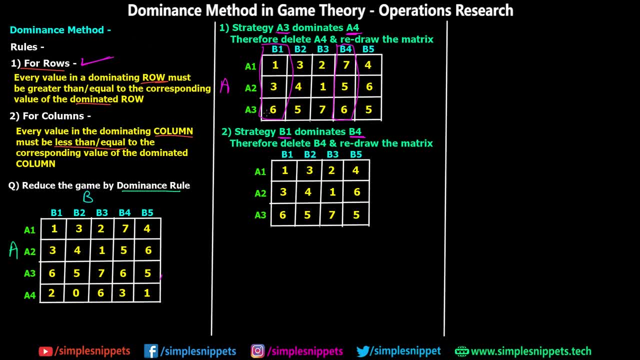 why B1 is dominating B4? because every value in B1, that is, 1,, 3 and 6, is less than or equal to the values in B4. So 1 is less than 7, 3 is less than 5 and 6 is not less than 6. 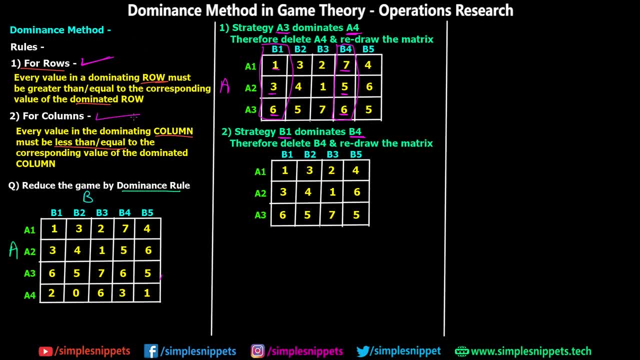 but it is equal to right, so even that is allowed. So that's why we're using this rule, And once we say that B1 dominates B4, we can completely erase out B4. So when we redraw the matrix, we don't have B4 in this new matrix. Okay, so I hope you're getting up until now and 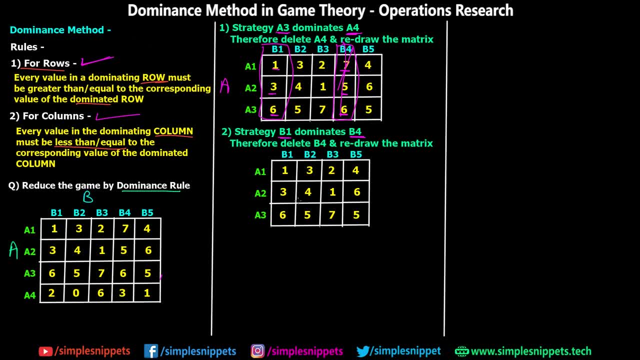 this is the same thing that we have to follow. You have to look for the dominating rows or dominating columns, whichever you find first, and then remove the dominated row or dominated column. So let's see step number three. So in step number three we say: strategy B2 dominates. 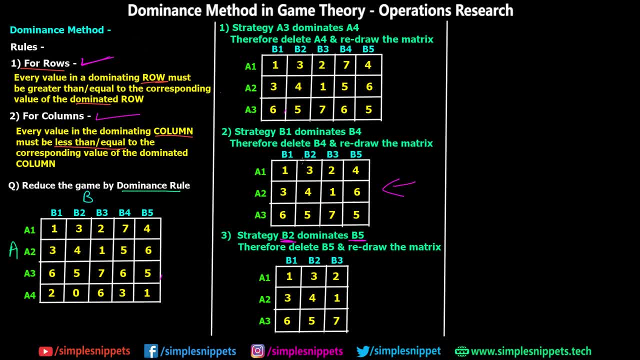 B5.. So from this resultant matrix you can see all the values in B1, B2, B3, B4, B4, B5, B2, that is, 3, 4 and 5 are less than or equal to B5. right, because 3 is less than 4, 4 is. 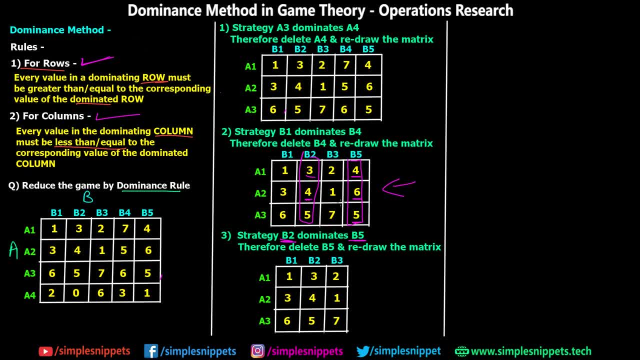 less than 6 and 5 is not less than 5, but it is equal to 5, which means B2 dominates B5 according to this rule for columns. So we can completely exclude B5 and rewrite this entire new matrix. So we've excluded B5 and now we have a 3 x 3 matrix. So let's see what. 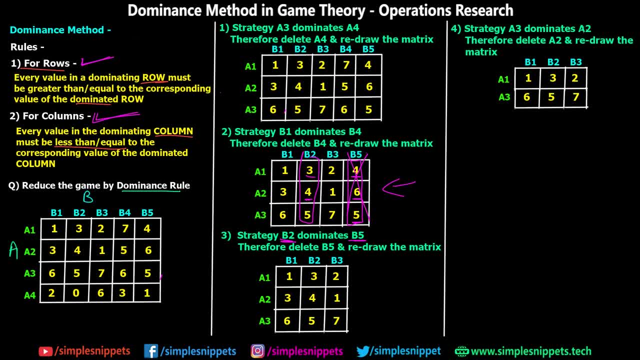 happens in step number four. In step number four you can see that A3 dominates A2.. So all the values in this row Are greater than all the values in A2.. So 6 is greater than 3,, 5 is greater than 4, 7. 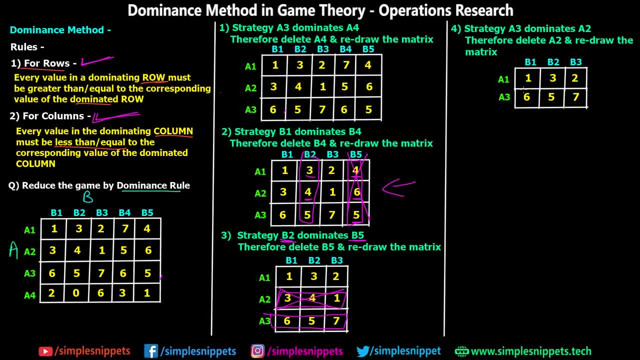 is greater than 1.. We can completely exclude A2.. So we erase A2 and we redraw the matrix. Moving on to step number five, you can see that A3 also dominates A1.. All the values in A3 are greater than A1.. 6 is greater than 1,, 5 is greater than 3 and 7 is greater than. 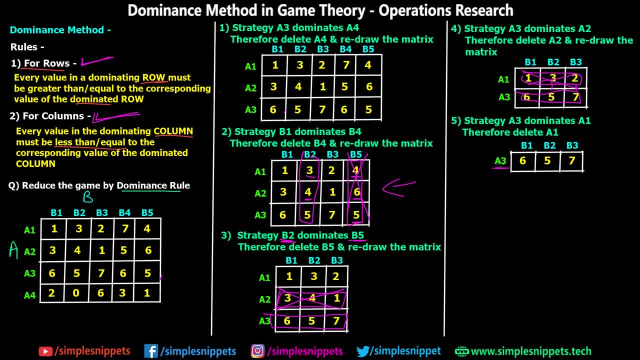 2. So completely exclude out A1.. So we are left out with only one strategy for player A, that is A3, and we have three strategies for player B. So let's see How we can reduce these strategies: B1, B2 and B3.. Now to reduce strategies of player. 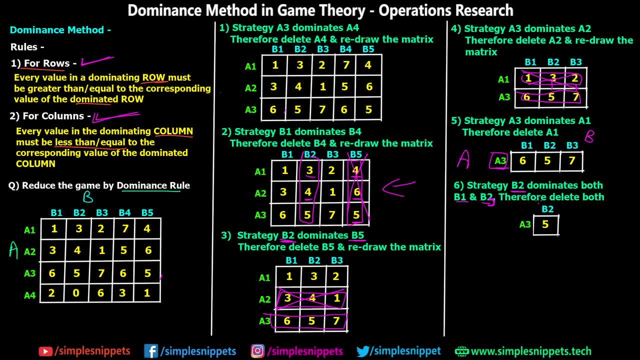 B. you can see that strategy B2 dominates both B1 and B3. So B2 has a value of 5, which is less than B1, that is 6, and it is also less than 7.. So you can completely erase out B1. 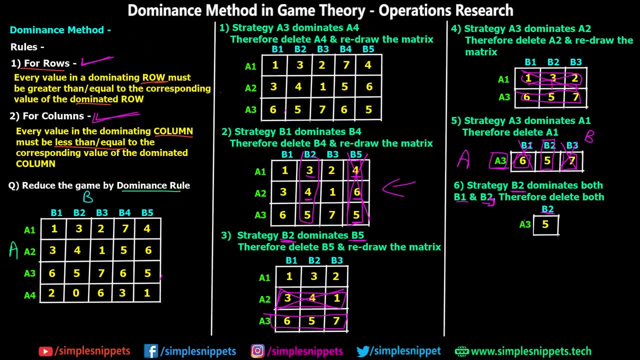 and B3 also, So we are only left out with B2 now. So this is basically our final answer, and we've reached our final answer and this is how you conclude the answer. So the value of the game that we've reached is 5.. 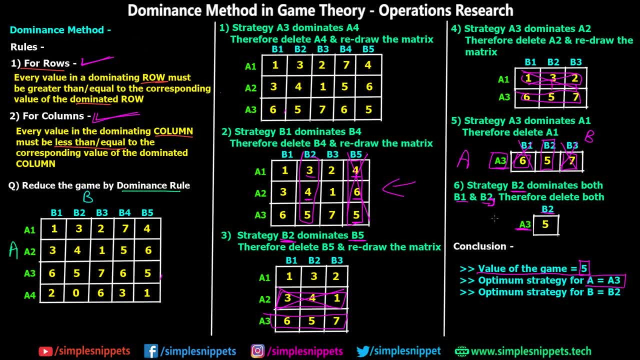 Optimum strategy for A is A3 because we are left with strategy A3 for player A. Optimum strategy for B is B2, because we are left with strategy B2 for B. So this is our final answer, using dominance method. Now, in this specific numerical, we could use dominance method completely. 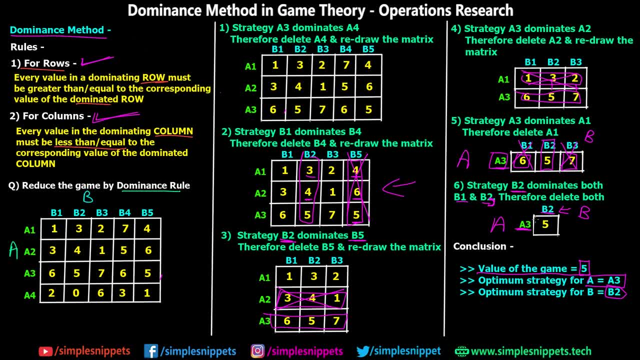 and we reached our final answer. but in most cases what happens is we use dominance method only to reduce the matrix to a certain level, after which we are not able to use the dominance method because none of these conditions become true, and then we have to use some other method. 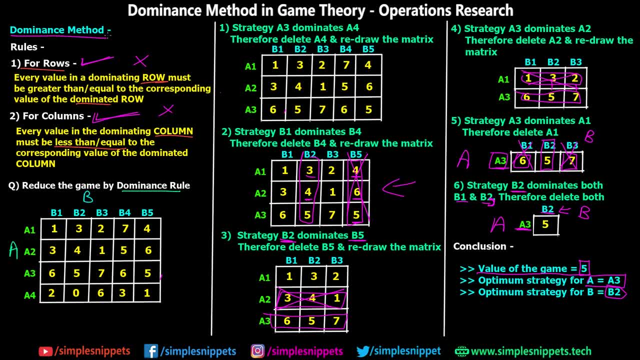 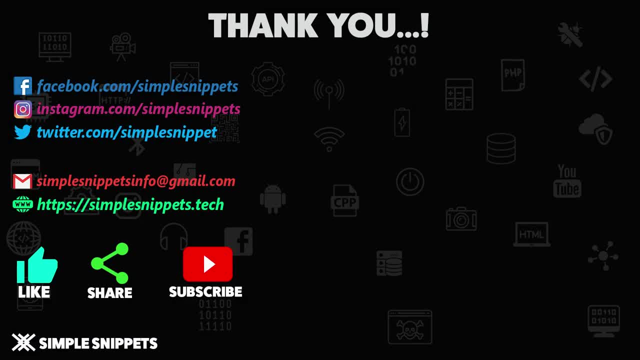 But since I just wanted to demonstrate the use case of dominance method, we took a numerical wherein the entire answer could be solved using dominance method. So that's it for this video, guys. In the next video we'll see some other method used to solve game theory and